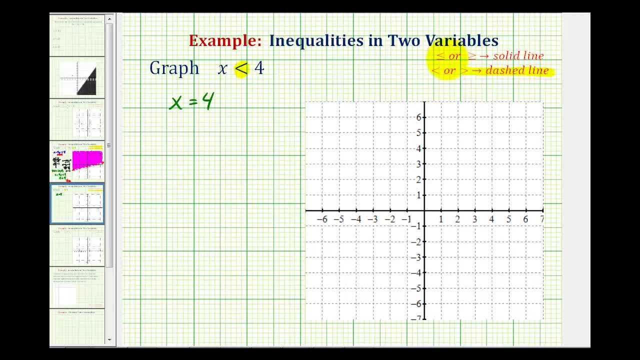 It's dashed because the line is not going to be part of the solution. If the inequality symbol was less than or equal to, or greater than or equal to because of the equal part, we'd have a solid line, meaning the line is part of the solution. 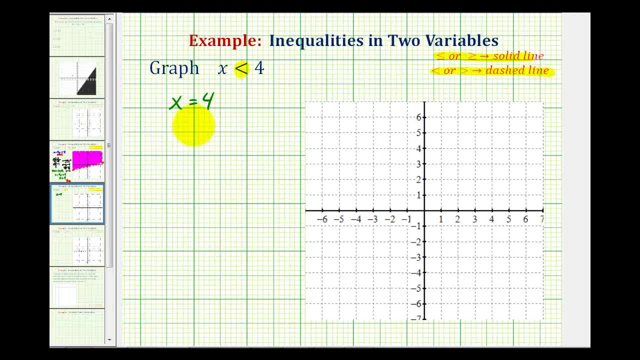 Just to make sure we know how to graph this line, let's complete a t-table and find at least two points on this line. This equation is telling us that x must equal four, So we can list four twice as an x-coordinate. This equation does not contain y, which means y can be any value that we want. 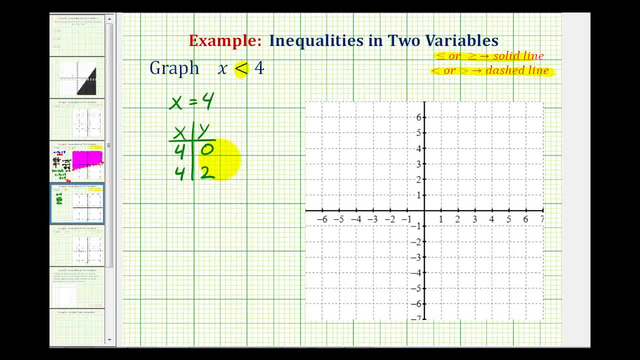 So let's say we have y equals zero and let's say y equals two. So we'll plot these two points and then make a dashed line through those two points. So here's the point four, zero, and here's the point four, two. 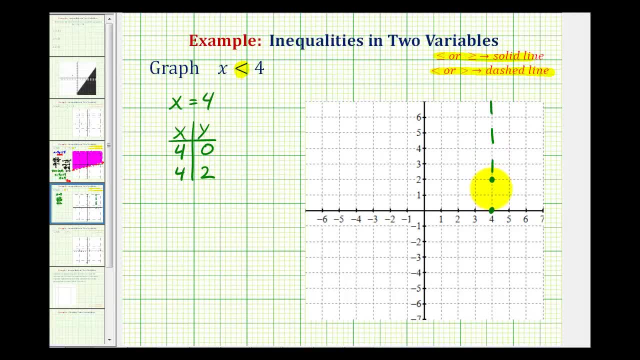 So we have a vertical line that's dashed that looks like this: Now, if you knew it was going to be a vertical line, that's great. If you weren't sure if it was going to be vertical or horizontal, I would always recommend making a quick t-table just to make sure. 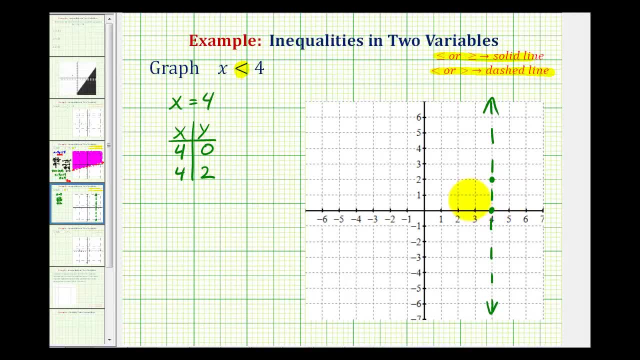 But now we need to check to see if we should shade to the right of this line or to the left of this line. But we should be able to figure this out pretty easily. if we can read this correctly, It says x is less than four. 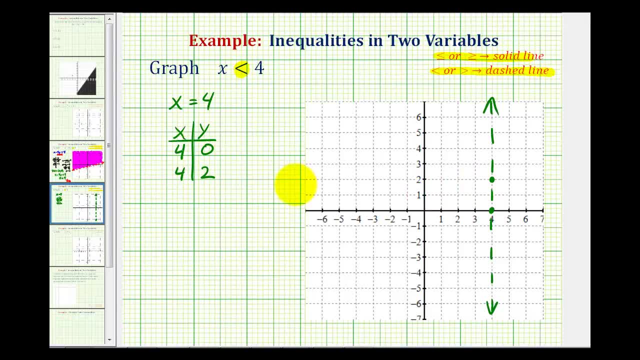 Well, x values are less than four to the left of this vertical line. So we'll shade the half-plane to the left of this line or this region here. Every point of this line is equal to zero. Every point in this region would have an x-coordinate that is less than four. 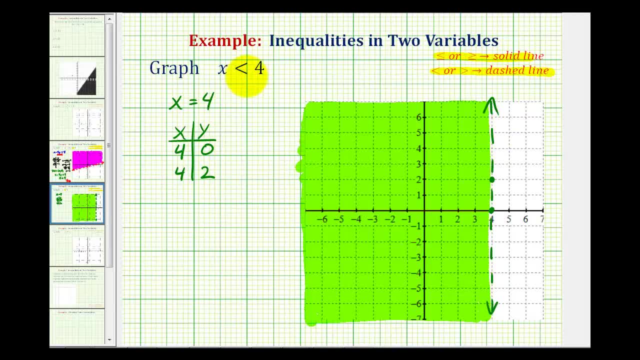 The line would contain all the points where the x-coordinate is equal to four and does not satisfy the inequality, And the points to the right. of this line contain all the points with x-coordinates greater than four or not less than four and therefore are not part of the solution. 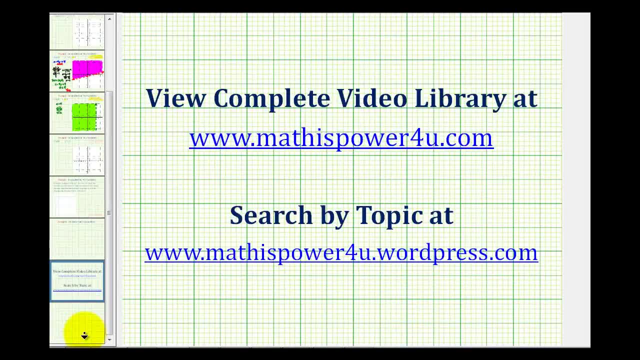 I hope you found this helpful. Thank you for watching.